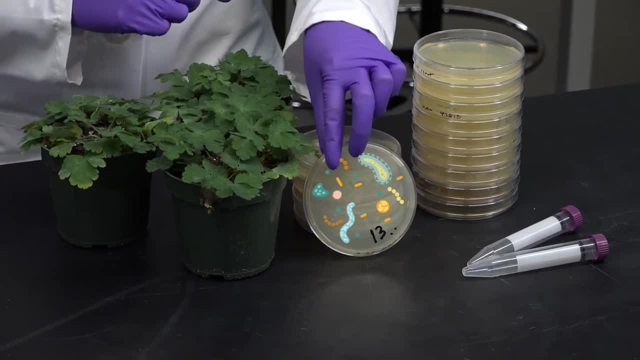 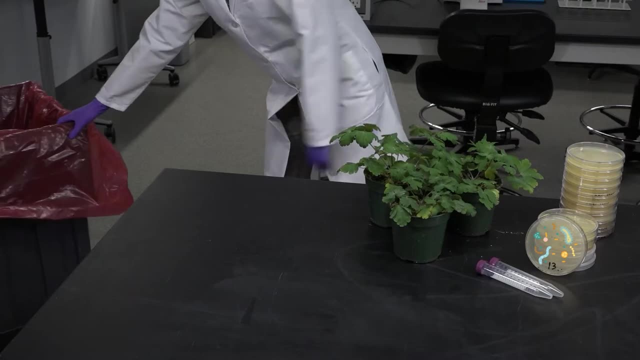 genetically modified plants, microorganisms growing on solid media and petri dishes, test tubes used in bacterial preps, etc. Solids can be disposed of in designated bio-waste containers. These containers are lined with a red bag stamped with the universal symbol for. 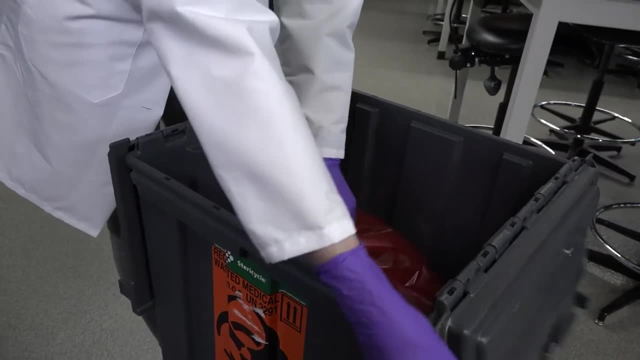 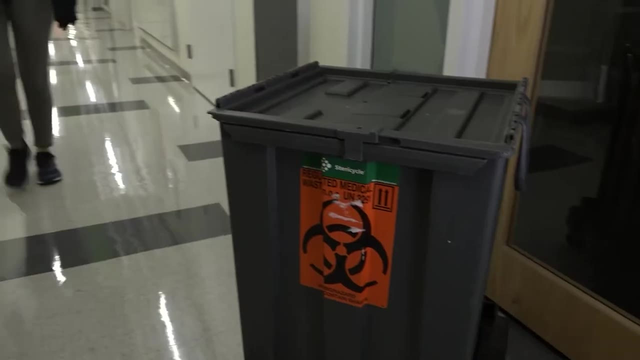 bio-waste. When they're three-quarters full, tie them with a single knot, close the bin and dispose of them according to EHS guidelines. In our case, we leave them outside our lab to be collected by trained personnel. The waste will be sent. 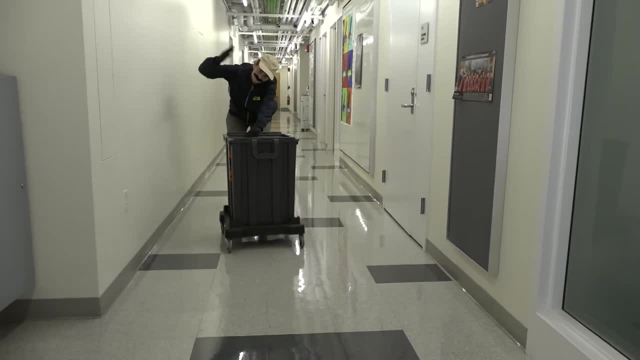 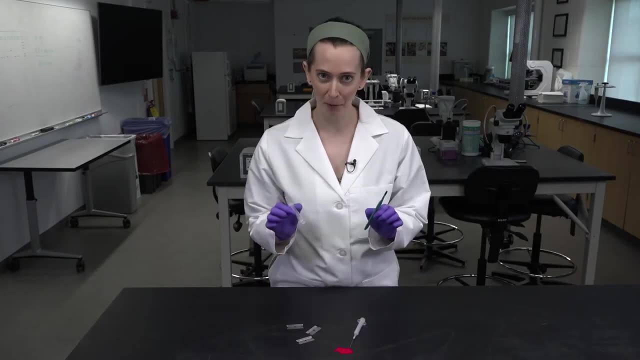 to a facility to be exposed to radio waves or incinerated to neutralize the biohazard before disposal. Because the solid waste is collected in plastic bags, you cannot put sharps like needles or blades in there. They'll poke right through the plastic, it'll leak bio-waste everywhere and it can harm the person. 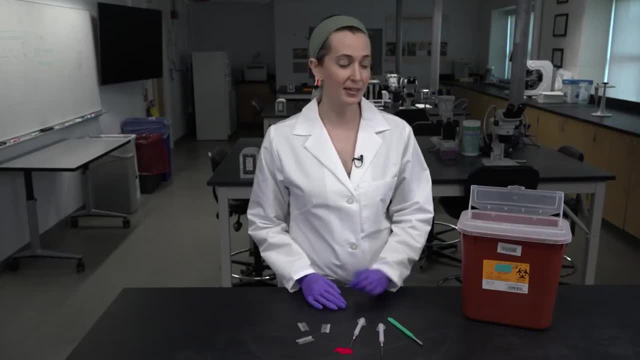 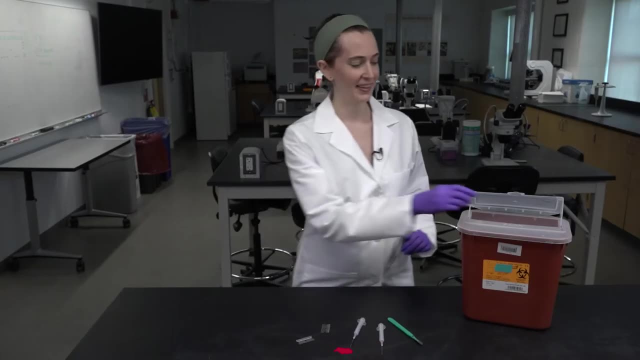 collecting the bags. Sharps contaminated with bio-waste need to go in special plastic containers that can't be punctured. They're usually red and stamped with the universal symbol for bio-waste. When they're three-quarters full, secure the lid and dispose of the sharps bin according to your EHS guidelines Here. 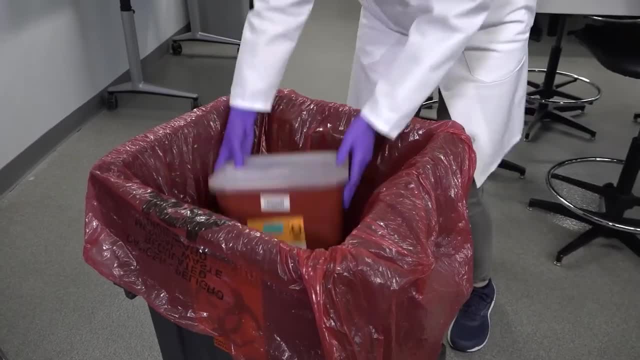 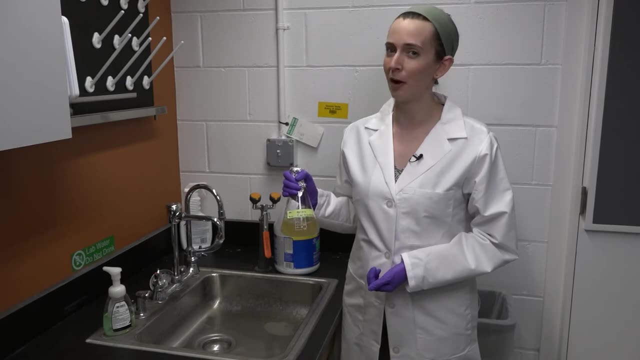 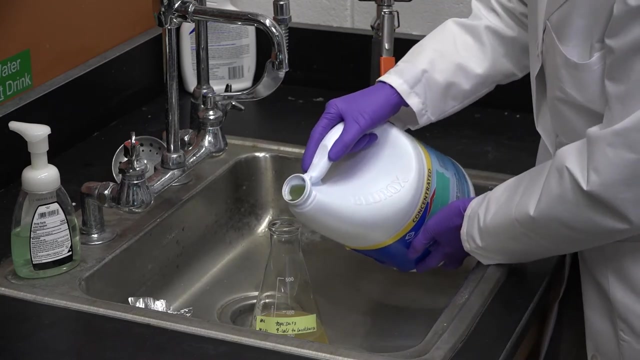 we can put the sealed sharps bin in the larger bio-waste container for solids. Liquid biological waste like these bacterial cultures needs to be treated with a chemical disinfectant before washing it down the sink. We add bleach to our liquid bio-waste to reach a final concentration of 10% bleach. So I have a. 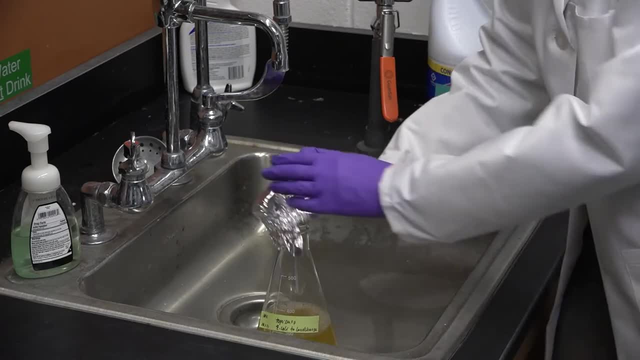 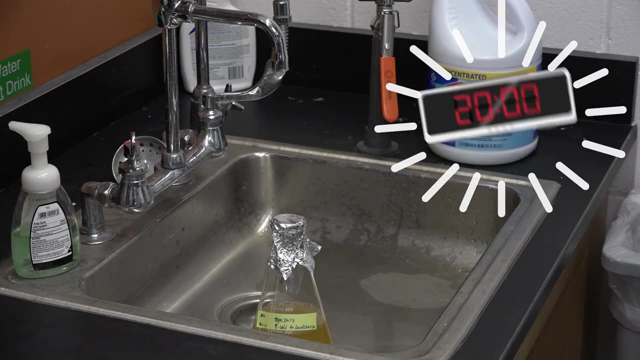 250 milliliter bacterial culture here, so I need to add around 30 milliliters of bleach. to reach 10%, The bio-waste has to sit with the disinfectant for at least 20 minutes before rinsing it down the drain with plenty of water When the 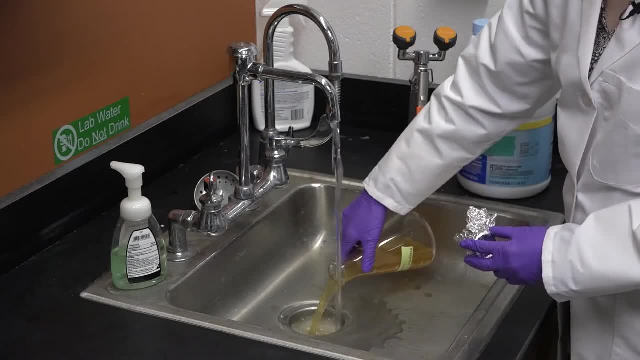 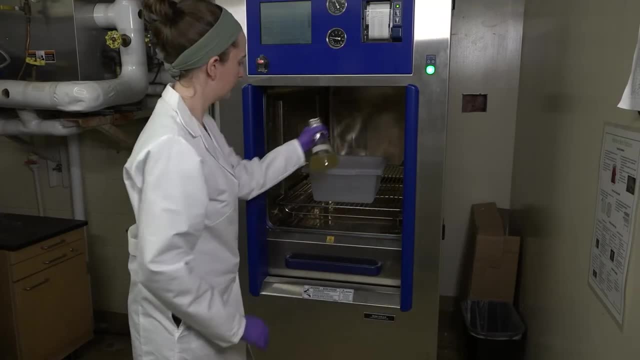 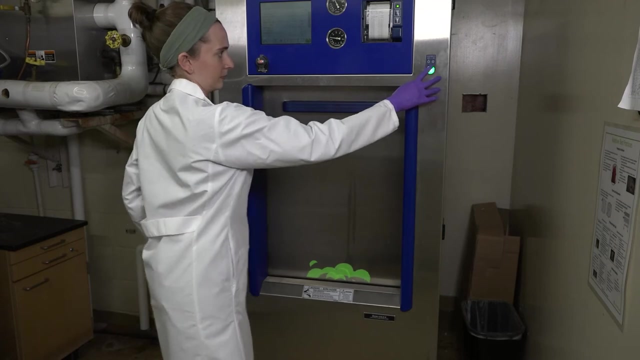 liquid bio-waste is completely dry, it needs to be washed down the sink. You can also autoclave liquid bio-waste prior to drain disposal, but do not add chemical disinfectant if you plan to autoclave. Bleach plus autoclaves equals very, very. 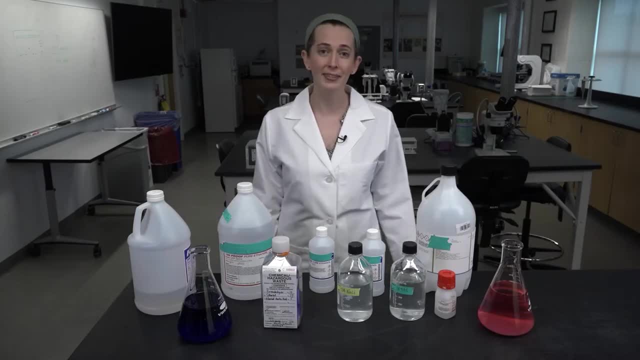 bad. Next, let's talk about chemical waste. Some of the chemicals we use in the lab are harmless and considered non-hazardous, like sodium chloride solutions or TAE buffer. These can be washed down the sink and non-sharp solids that have come into contact with them can be put in the. 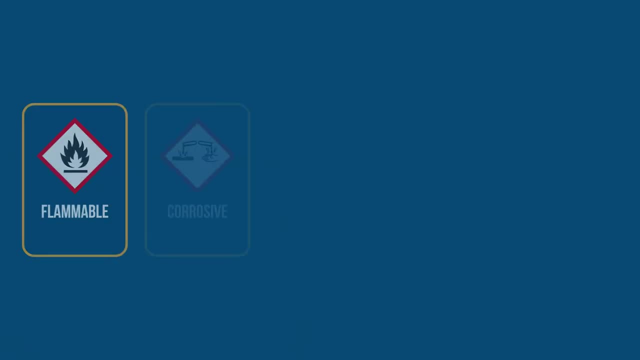 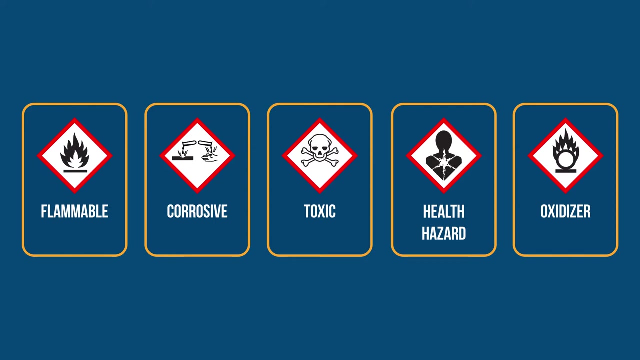 regular trash. But many other chemicals are considered hazardous because they're either flammable, corrosive, toxic, an oxidizer or some combination of these hazards, and they all need to be disposed of according to EHS rules. You should follow your institution's protocols, but here are some general guidelines. First, 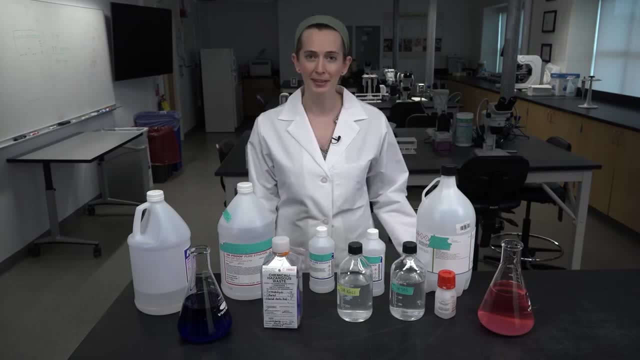 it doesn't make sense to call EHS to pick up your chemicals every single time you do an experiment, because often you don't have enough time to do that. So when you're working with really small volumes, you can't be like. 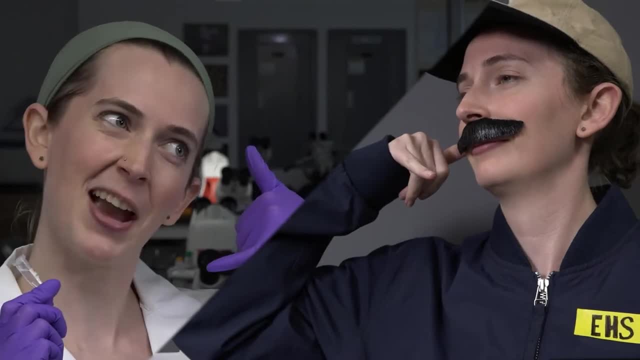 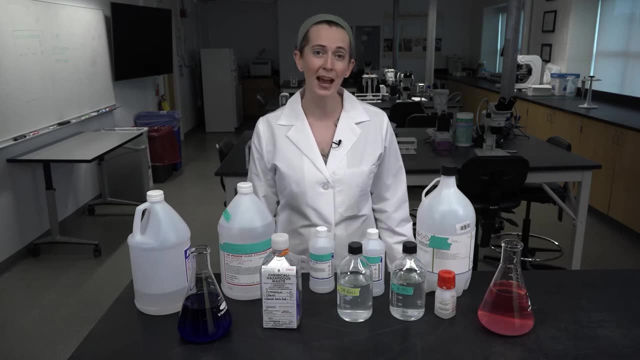 Hey, EHS, I've got one milliliter of formaldehyde for you. can you come and get it? Instead, labs maintain collection bins for hazardous chemical waste, so you can add to them over time and just call EHS when they're getting full. These waste bins have to be. 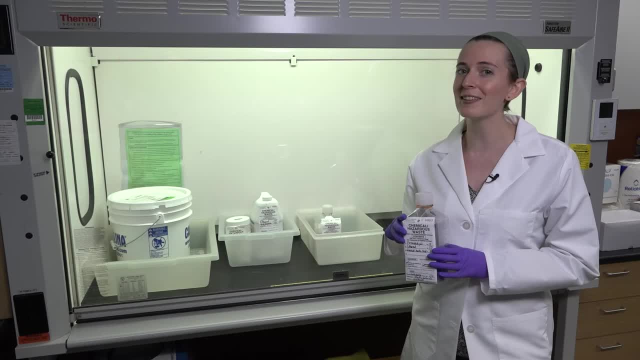 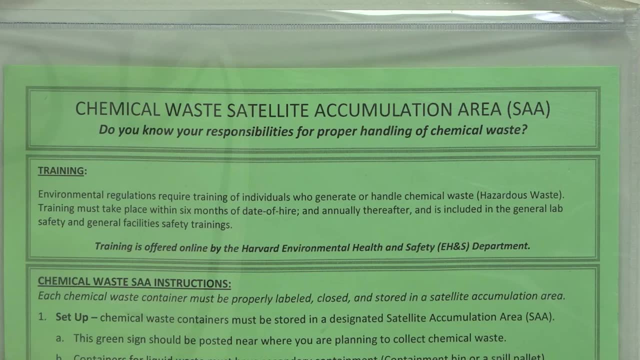 stored in specially designated areas of your lab, called chemical waste satellite accumulation areas. They're typically located in the fume hood so that fumes from the waste can't leak into the lab. They don't have to be stored in secondary containers like those plastic tubs, and they 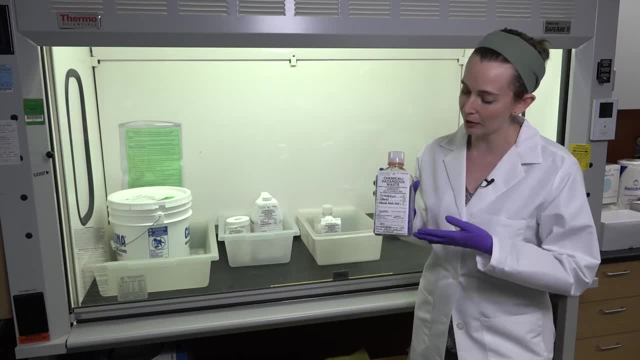 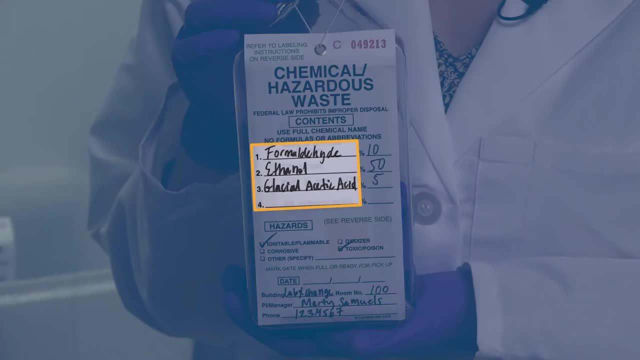 have to be labeled according to EHS rules. Let's take a look at a label for a common tissue fixative- FAA. First notice: the label doesn't just say FAA. You need to spell out the full name of the ingredients it consists of, In this case, formaldehyde, ethanol and. 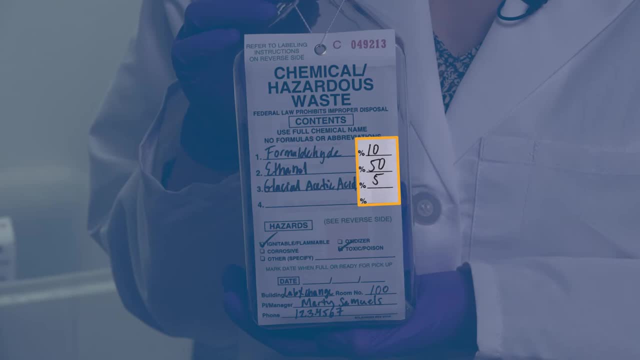 glacial acetic acid, as well as their respective percentages, what types of hazards they confer, where the container is being stored and the type of waste they're storing. If you have a label that says FAA, you have to take a look at the label for a common tissue. 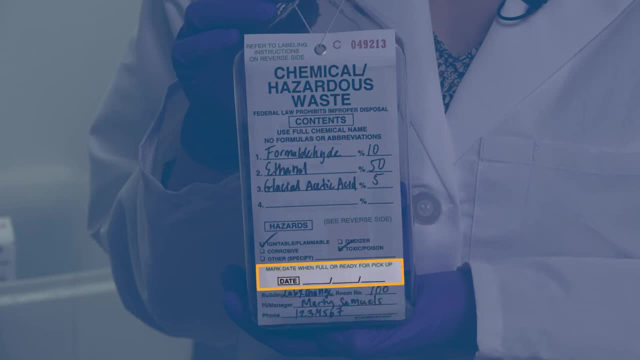 fixative and the contact information for your lab. Notice: we don't fill out the date right away. We only do that when the container is full and we've scheduled a pickup, because it's actually illegal for waste containers to hang out for more than three days after dating the tag. 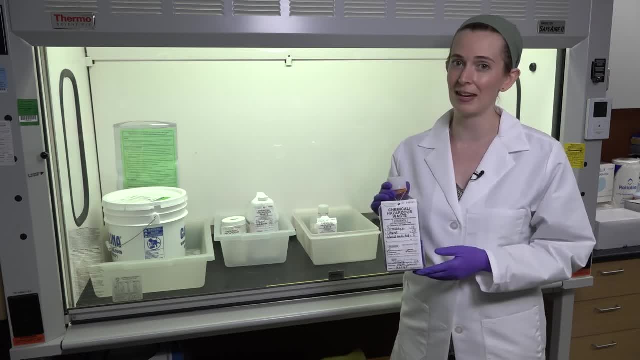 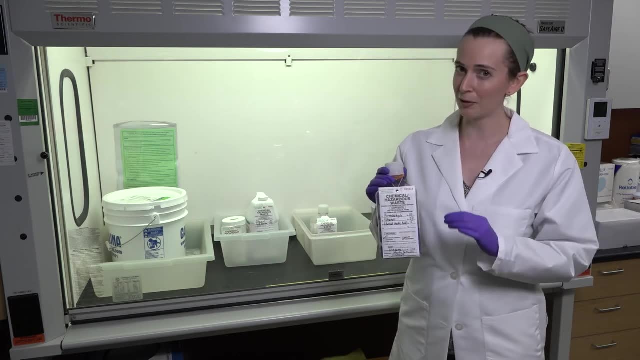 Liquid and solid waste for a given chemical can often be combined in the same container, but check with your EHS office first, as protocols can vary. Combining different chemicals into one container is generally not recommended, though You know, of course, FAA already consists.